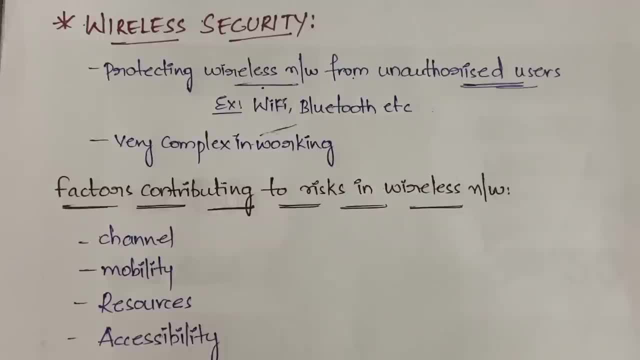 wireless devices like. it can be anything. it can be a wi-fi router or it can be a bluetooth device. it can be wireless headphones, wireless, you know, it could be airpods or it could be anything. it could be anything, any wireless device. we have to protect that. that is what wireless security is. 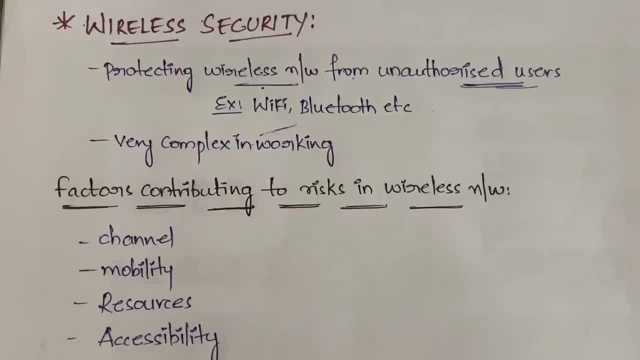 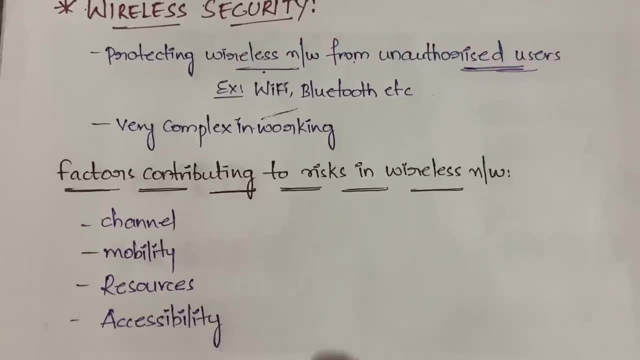 and it is very complicated in work because, since there is no end-to-end connection between that, there is no physical wire, physical connection between that. so it is very complicated. now let us see what are the factors that are contributing to the risks in the wireless network. first is the channel, the channel through which 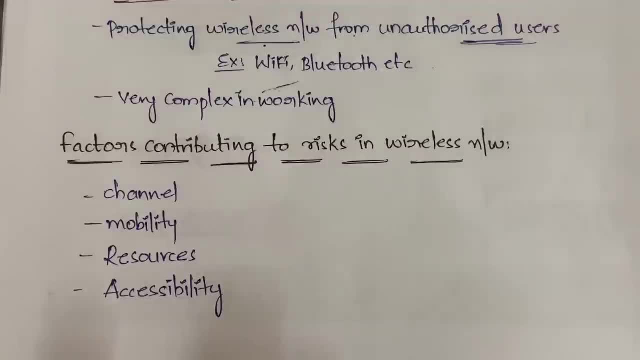 communication is taking place and the mobility that is. you can- uh, you know- shift the devices right. you can transfer the devices from one location to other location. you can take your uh bluetooth headphones or you can take your airpods. you know, you can shift them from one. 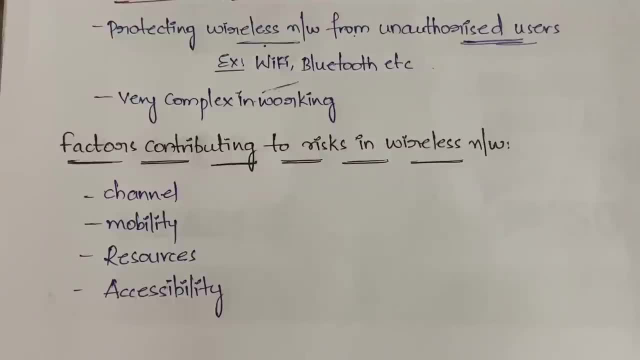 location to the other location. all these factors are contributing to the risks of the wireless network. now let me end this session with some oil and resources and the accessibility. so these are the different factors which are contributing to the risks of the wireless networks. now let us see what are the different threats. 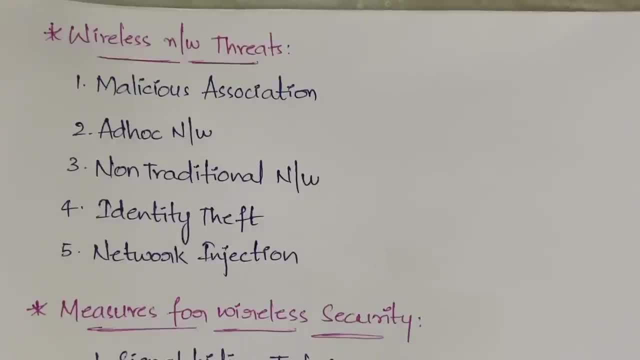 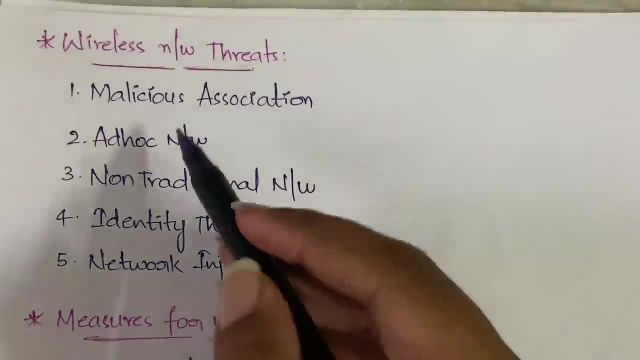 of the wireless networks and how to overcome those threats. now let us see what are the wireless network threats, that is, uh, what are the possible threats, these kind of threats maker, and not only these. there are still more. but uh, we will, you know, generalize some general threats. we will be. 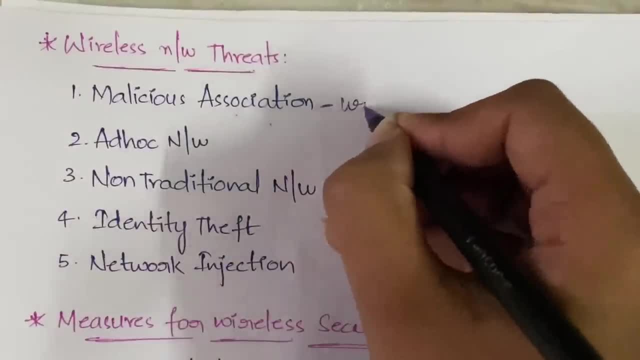 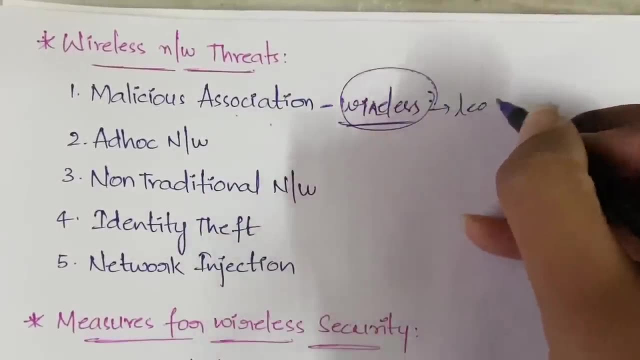 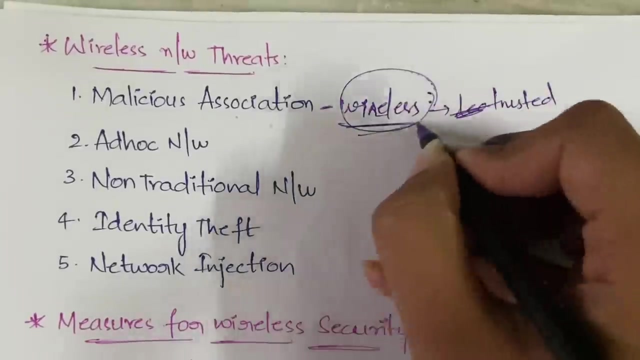 you mean by malicious association is a wireless device. you will have a wireless device and this wireless device is configured in such a way that it appears to be a legitimate device- legitimate otherwise. i'll tell you in a simple word: um, like you know, trust it. it appears to be, it is. 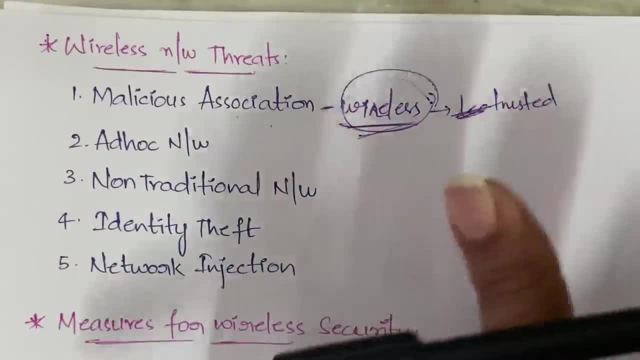 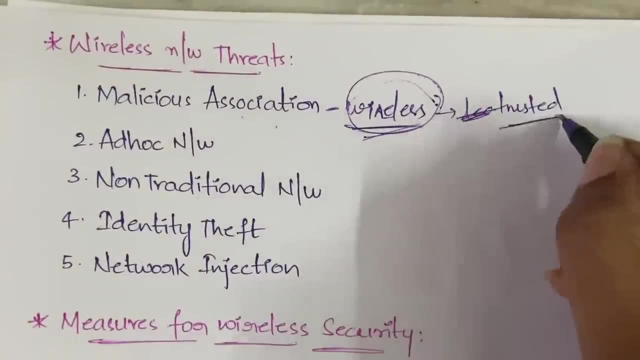 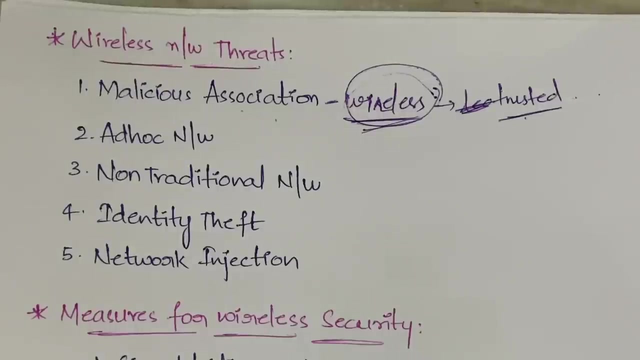 configured in such a way that to the user it will be appearing as a trusted device only. okay, but actually it is not right. so the user will think that, okay, it is a trusted device, so i can connect to it, so the user will connect to it and all the data will be stolen. okay, so this is what malicious 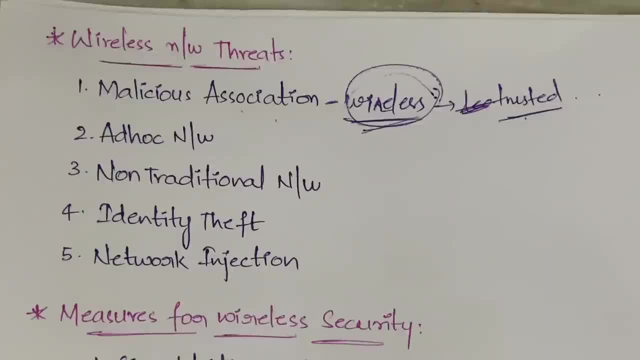 association means a wireless device will be configured in such a way that it appears to be a- you know, a trusted source to the user. the user will think that, okay, it is a trusted device, or it is a trusted network, or is it is a trusted connection and the user will get connected. 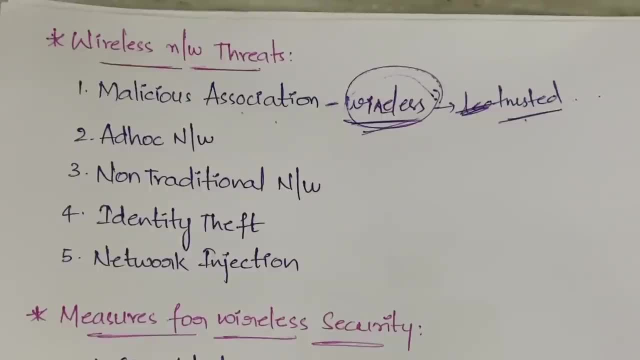 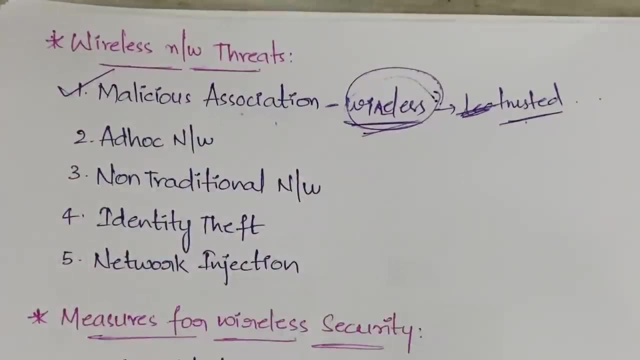 to it. so once the user gets connected to it, all the data which is related to the user is stolen by the third party. got it. and next comes the ad hoc networks. ad hoc networks are nothing but the wireless network. right, you know what are ad hoc networks. i hope ad hoc networks are also wireless networks. 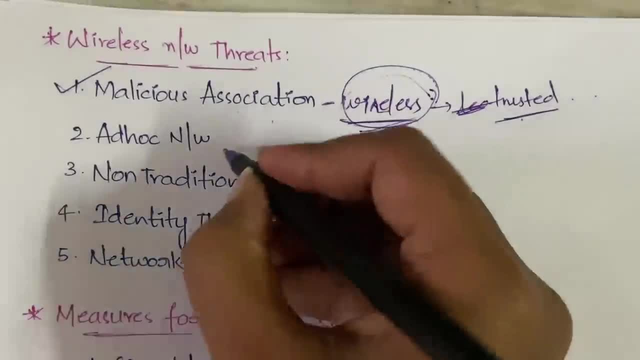 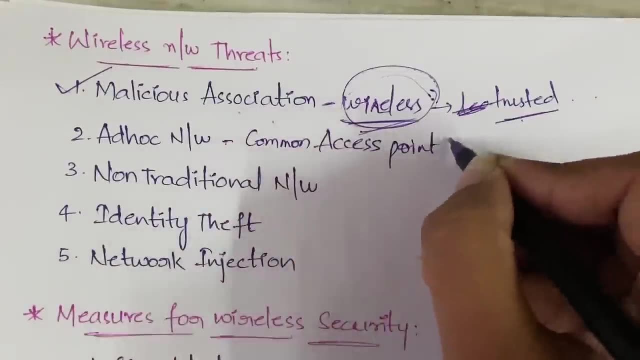 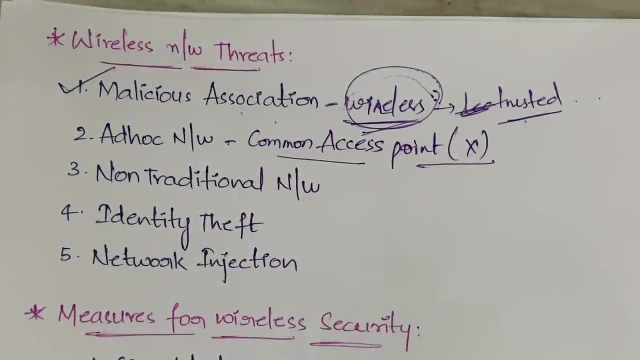 and they, you know they don't have access in the sense they don't have common access point between them. they don't have a common access point, no common access point. so because of that reason, there may be no security between them, because there is no common point to communicate. uh, or you? 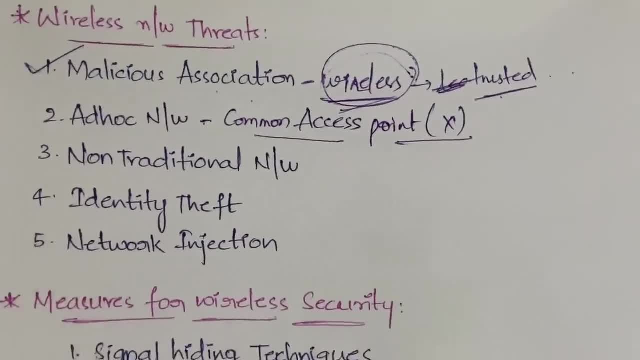 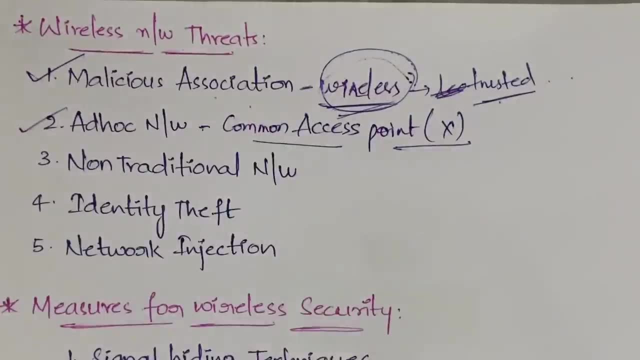 if, if, suppose, if, if at all, you identified a threat in the network, then you can communicate it to the others. right, but in case of ad hoc networks, since there is no common point to the devices or networks, so there is a more chance of security and non-traditional networks. non-traditional 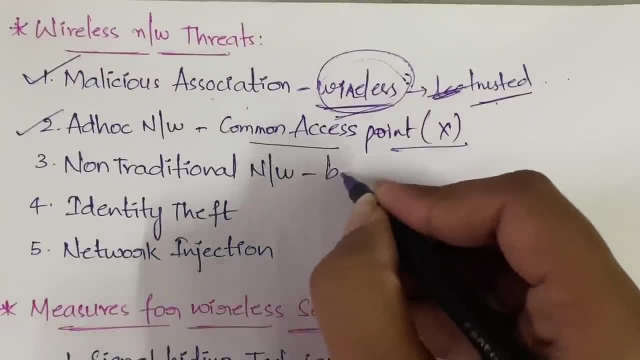 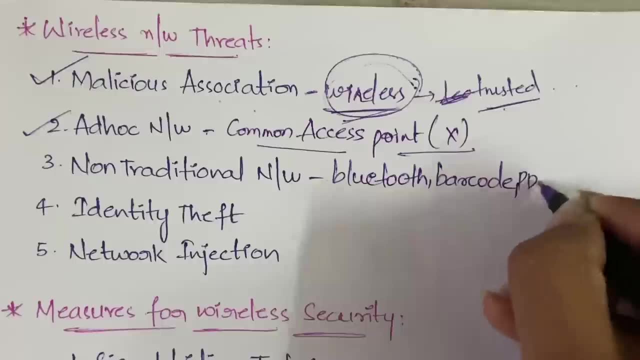 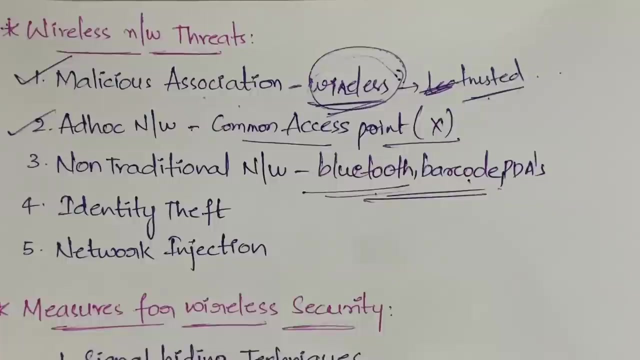 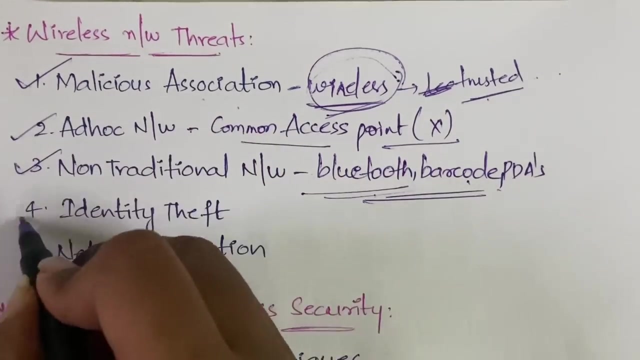 networks are nothing but um. you can say bluetooth, bluetooth and barcode readers and pdas- all will come under the non-traditional network, since they are also wireless. bluetooth is wireless, right? barcode reader is also wireless. so since the all of them are wireless, so they do not have much security. next is identity theft. so 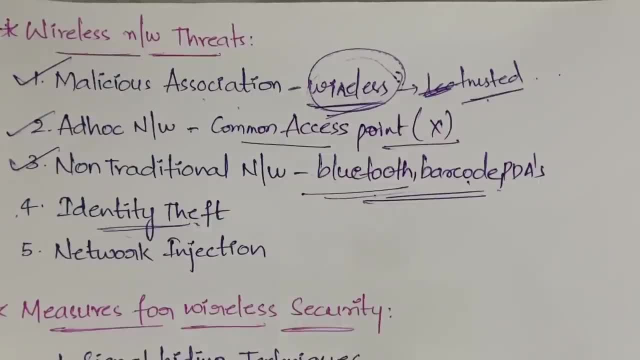 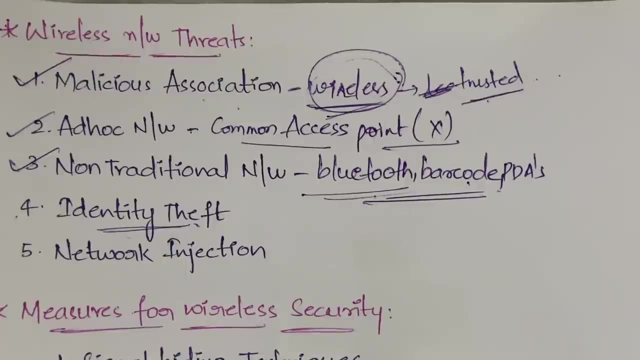 see, for any person, identity is very important, right, even for everything. also, each and everything, each and every uh food item or any clothes or whatever you buy, will have a unique barcode with on them. so, in the same way, even an identity is very important for the computer as well. 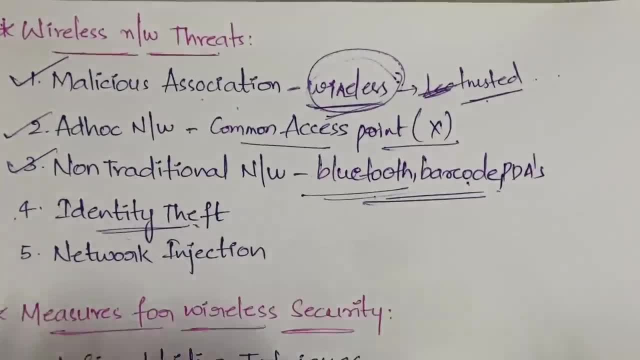 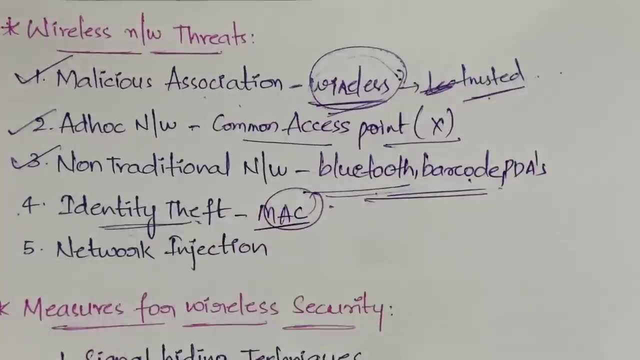 so here what happens is the attacker will observe the network traffic and he will steal, he will find out the mac address of the computer. okay, so whichever computer is using the wireless network, so on that computer he will observe the network traffic. that is on google what you're searching. 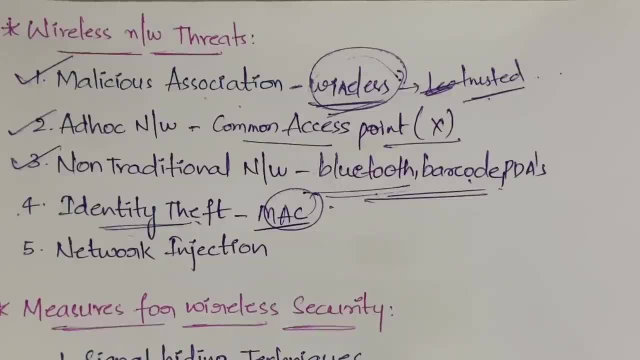 what you're doing, what login credentials you do. so all that will be observed by the attacker and that attacker will steal your data, will steal your mac address. mac address is obviously an important factor to the computer. so you have to remove those scriptures manually and get rid of those such things. 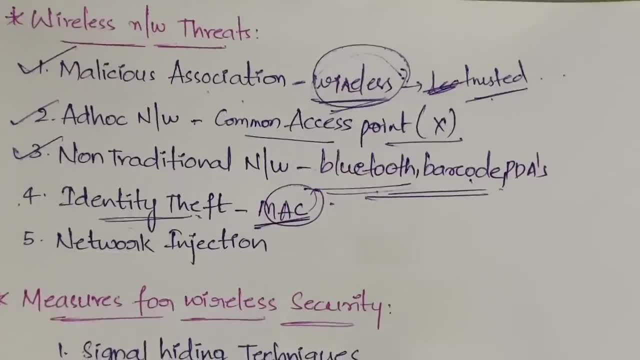 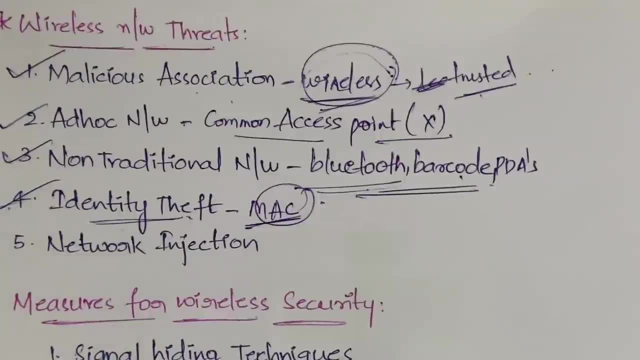 right. so obviously, if your mac address is stolen, your computer is at risk. next, network injection. so network injection, in the sense you will be some, you know, so much of data will be injected into the network without the users. user will not know that the data is being injected into the. 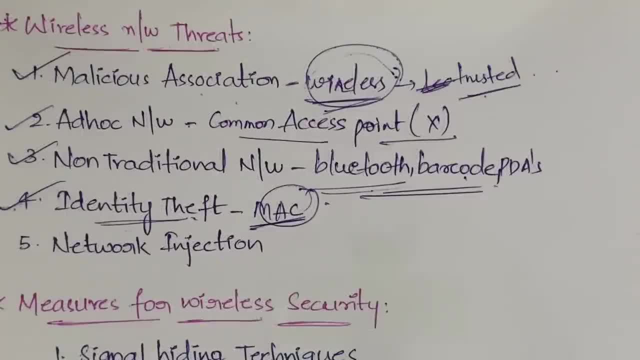 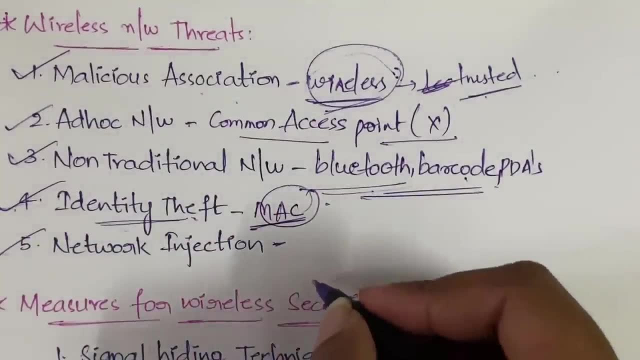 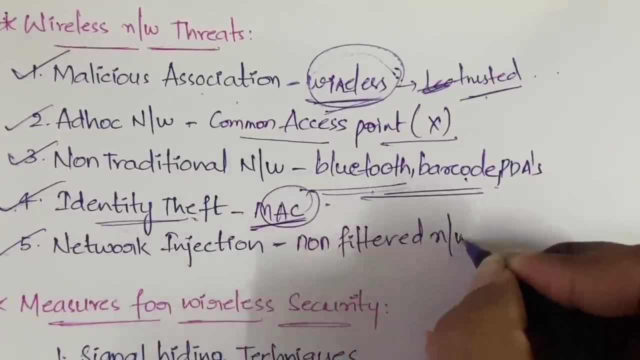 network without the users or users notice, the data will be injected and this will be this network injection mainly happens in the systems where you know the data. the systems are being exposed to non-filtered network traffic, that is, the traffic is not filtered. in that case, this network injection. 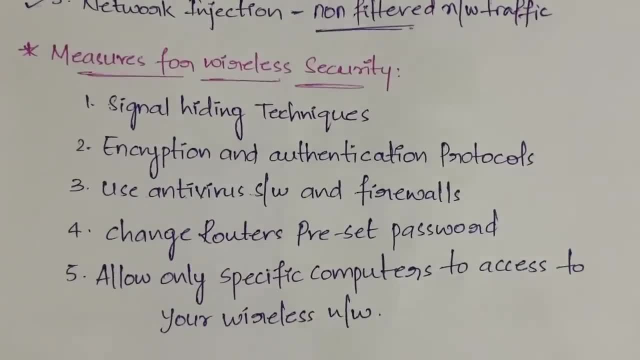 is very common to happen. got it, and now? what are the measures for wireless security? so measures, in the sense, what we have to do in order to ensure wireless security. this is very common. you already know all these things. so the first thing is signal hiding techniques. so what do you mean by signal hiding techniques? is 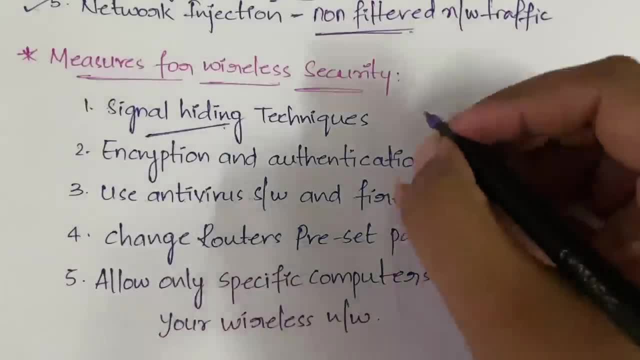 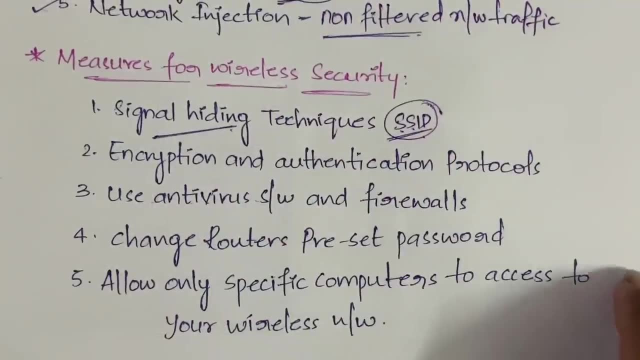 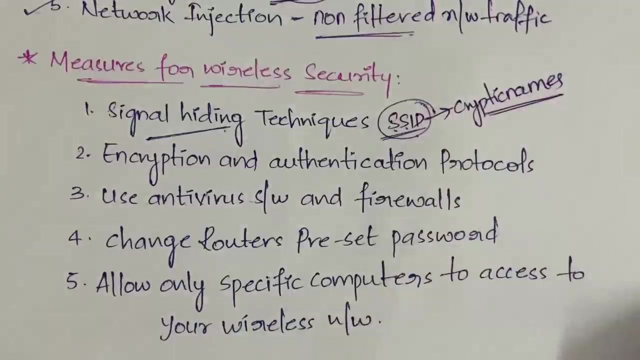 nothing, but you need to turn off the service set identifier. it is ssid. the service set identifier, ssid, has to be turned off, okay, and also you have to assign cryptic names to them. cryptic names is nothing but some names which cannot be understood, right? some random combination, like you know: s b? u. 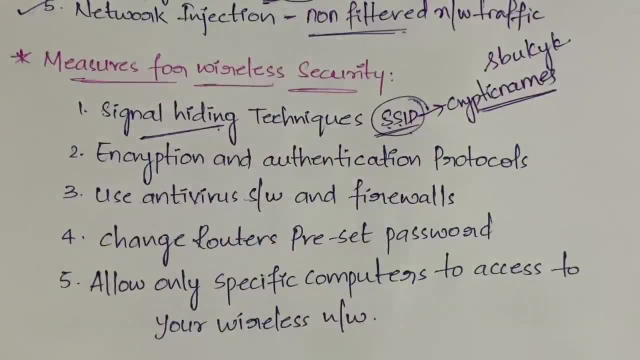 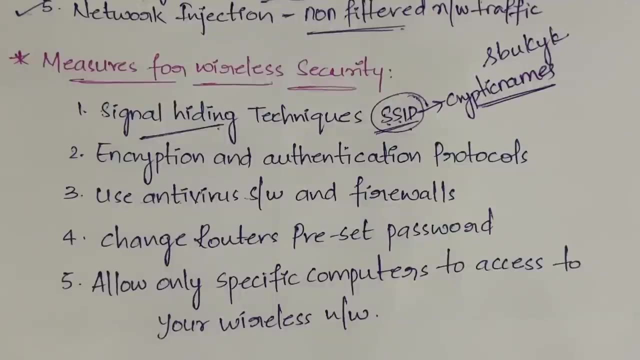 k, y, like that. some random generation, some random thing has to be assigned so that it is hard to remember, it is hard to identify, it is hard to guess. also got it. next. you have to reduce the signal strength to the lowest level. that is how much ever possible level you can lower it. you can suppose in an office, in a floor, suppose there. 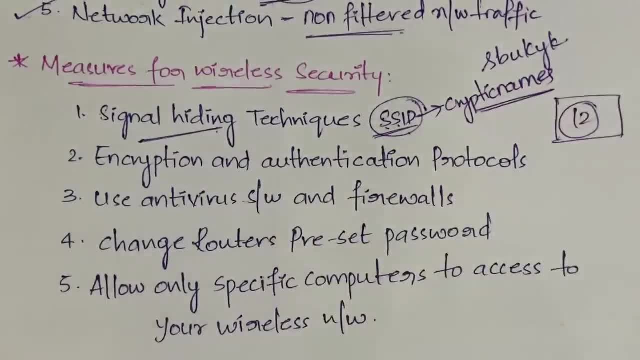 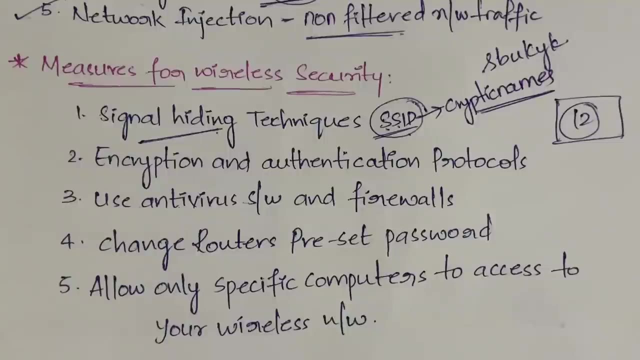 are 12 employees working right. so you have to reduce the signal strength so that the it has to be sufficient only to 12 employees, not more than 12. got it. the signal strength has to be lowered. at the same time, the low signal strength has should not be a problem to the users who are using it. 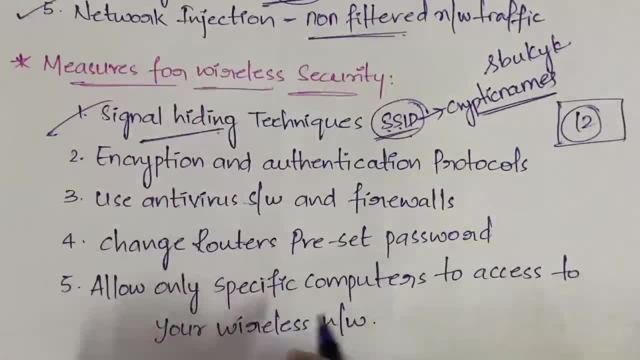 got it and yeah, that's all, and you can also. yeah, one more thing: you can also locate wireless access points, like any wireless routers or wireless, any wireless access points inside the building, not outside of your building it. they should be located inside of your building and that. 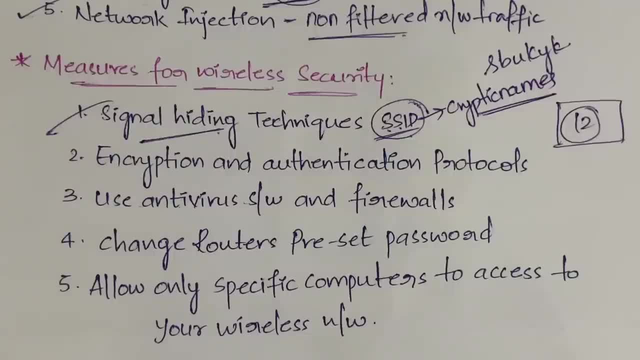 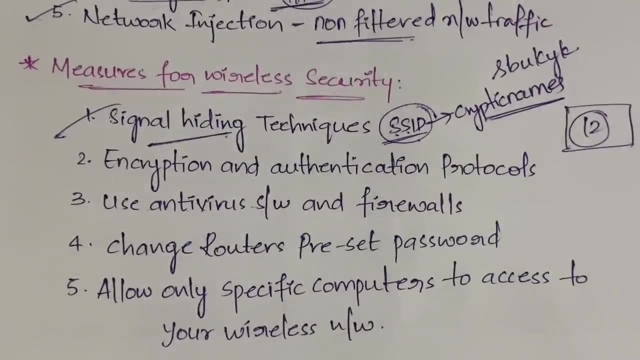 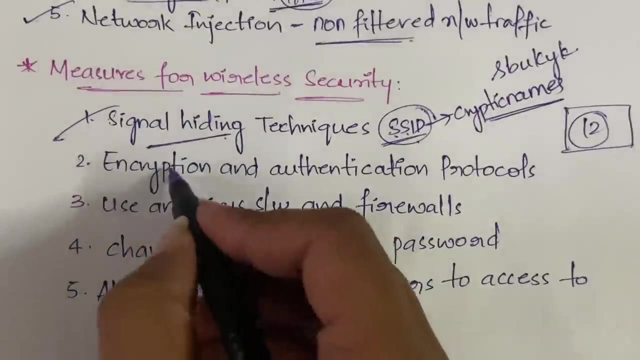 too, not closer to the windows or walls in the center of the room probably got it. so all that things you have to do in signal hiding techniques, all those things will come okay. next, encryption and authentication protocols. that is, you need to use some encryption and authentication protocols. you know what is encryption? right, plain text to ciphertext. 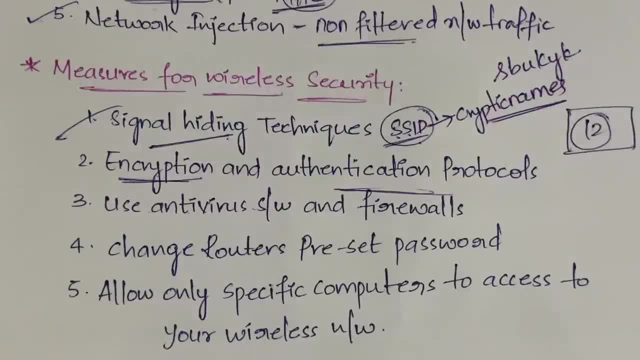 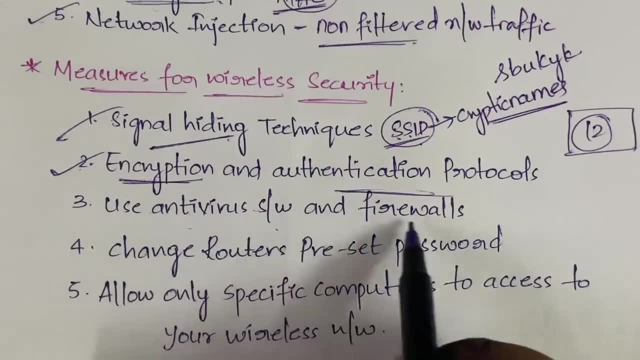 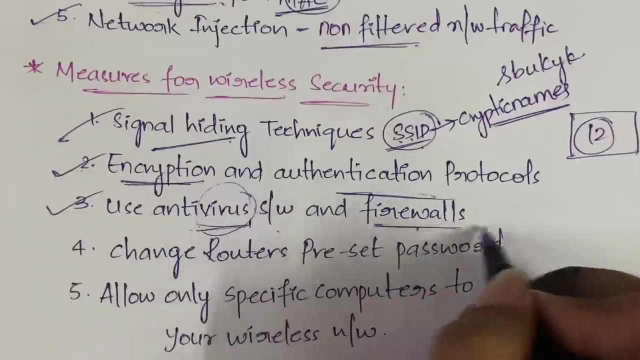 even authentication protocols also. you have to use very strong authentication protocol so that the data- uh, you know- cannot be easily identified by the attacker. next, use antivirus softwares and firewalls- you already know that- so that you don't have any virus into your computer. and firewalls also, to you know, prevent some untrusted data and change routers preset password. 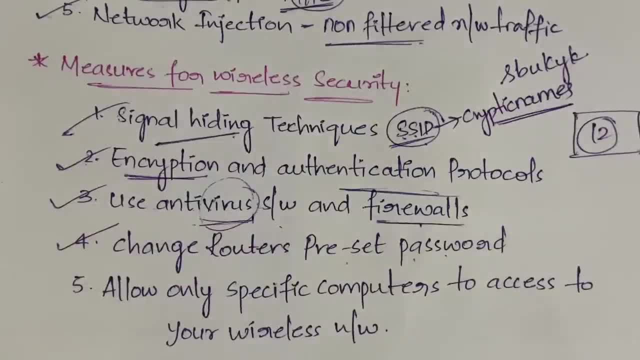 that is when you purchase a router. when, when or when an organization purchases a router, a router will have its preset password right initially. it comes with a password. you should not continue with that password. okay, you have to change and not only preset password for each and every uh. 60. 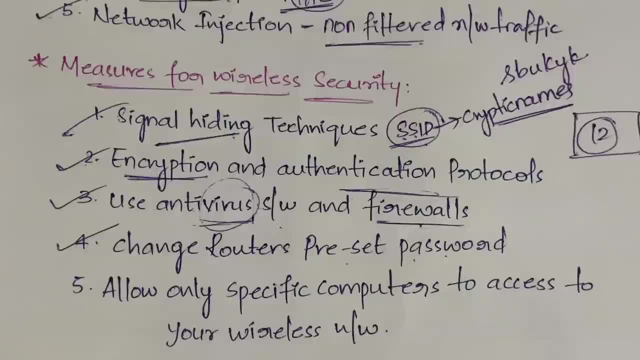 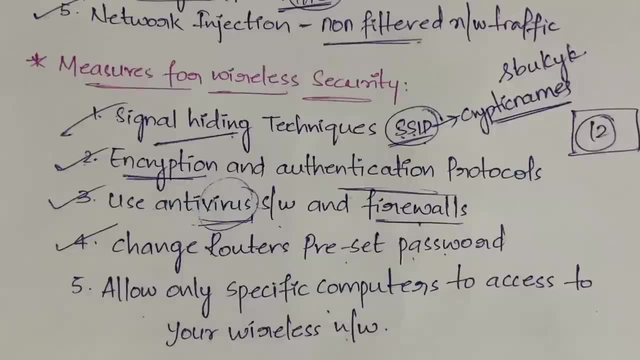 days or 75 days or 90 days. you have to keep on changing your passwords. okay, and next, allow only specific computers to access your wireless network. that is, you should allow only specific computers, not all the computers like, for example, um, for example, in your organization or 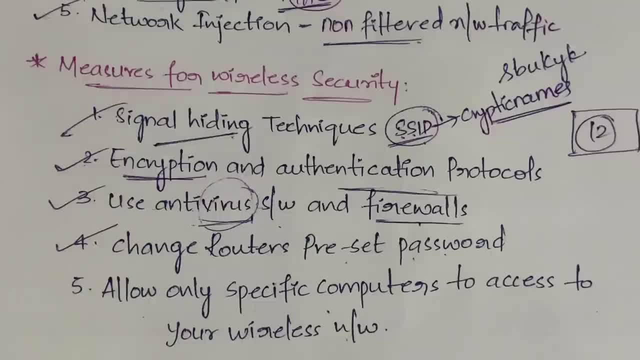 in an office or at your home, you're having your wi-fi. wi-fi is also wireless, right? so you are having your wi-fi network and you should not give- you will not give your wi-fi password to whoever comes and ask you. you will not give it to them, right? so whoever should use your wireless network? 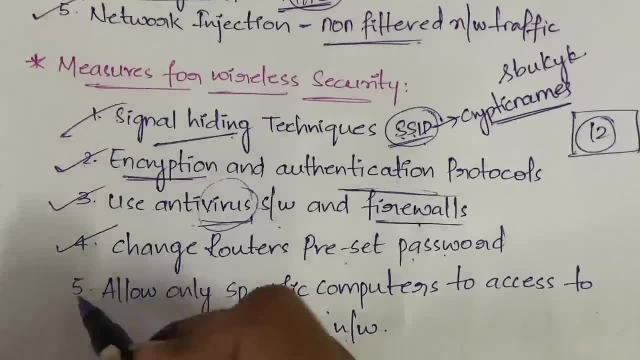 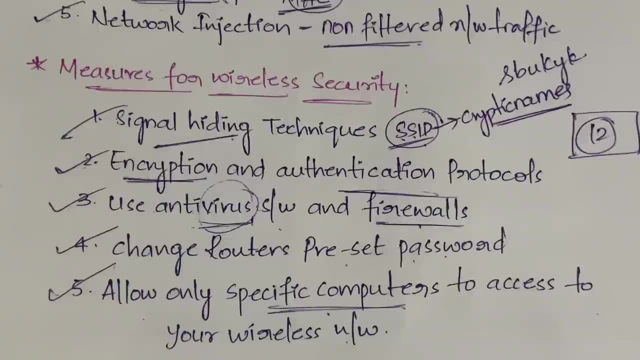 that has to be decided by you got it. allow only specific computers. do not give access to each and everyone. so that's all for this video, very simple, um, you just listen to this video. after listening to this video, you can write everything on your own. there is nothing that you have to write the same side, headings and.